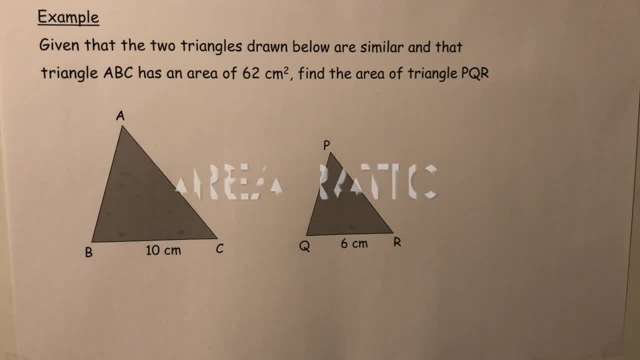 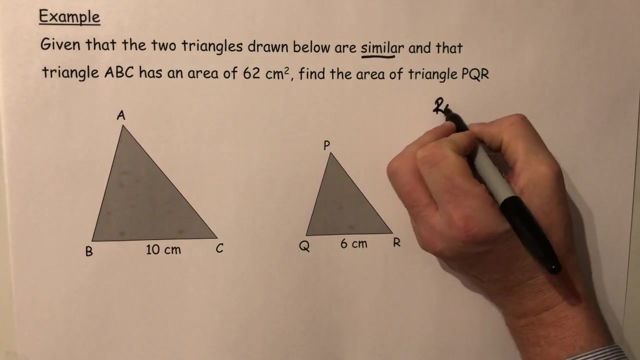 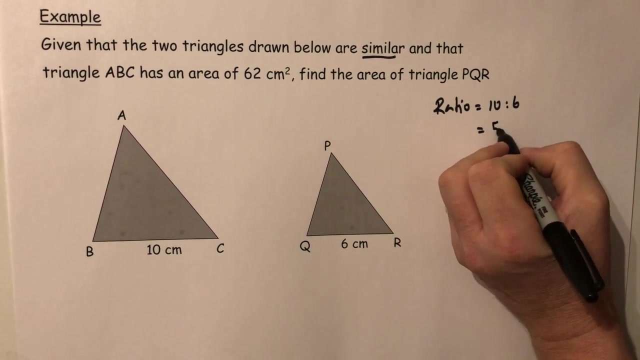 Now, in this particular question, we are told that these two triangles are similar. That means that the sides are in a given ratio, And we can see that this side here must therefore match with this side here. So the ratio of the sides is 10 to 6, which can simplify as 5 to 3.. 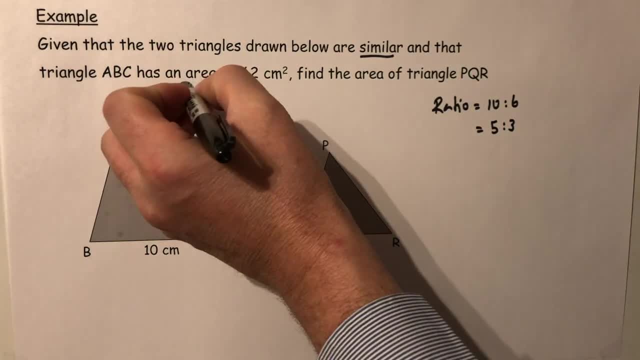 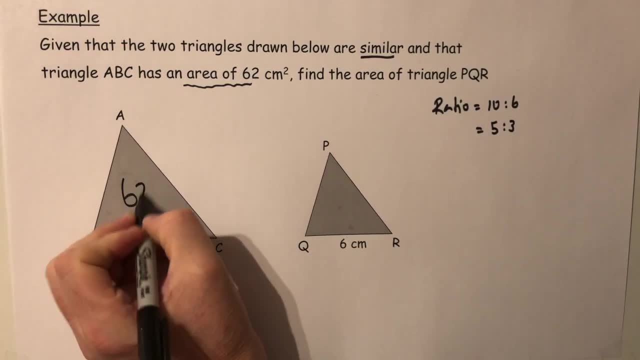 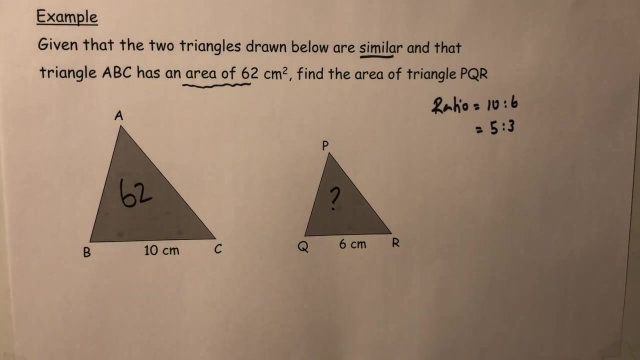 However, this question talks about the area, And we're told that the area of ABC, the area of that one, is equal to 62. And we're asked to find the area of this one. Now, what you have to recall here is that this ratio is for the lengths. 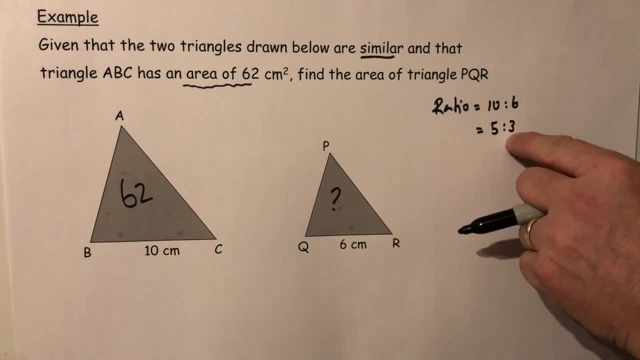 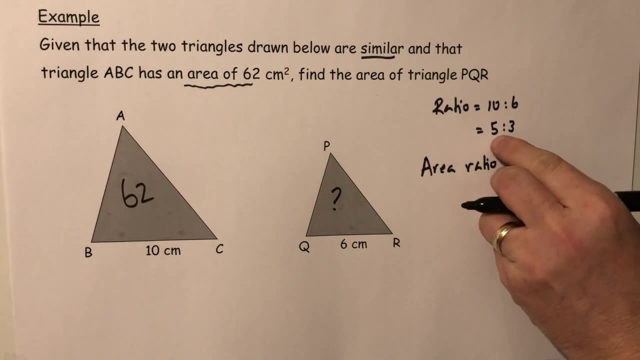 So the lengths are all in this given ratio. That means that the area is in a different ratio, which is 5 squared to 3 squared. Therefore, in order to find the area of this triangle, area of this triangle is equal to 6 squared. 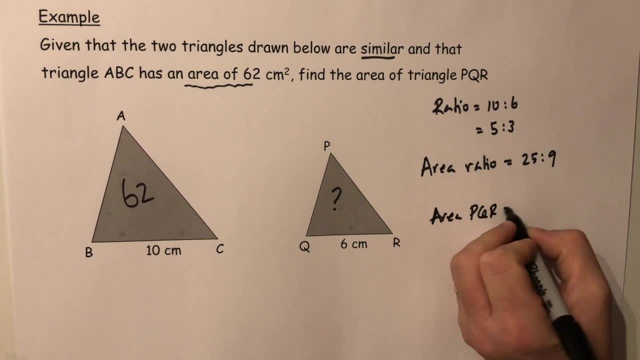 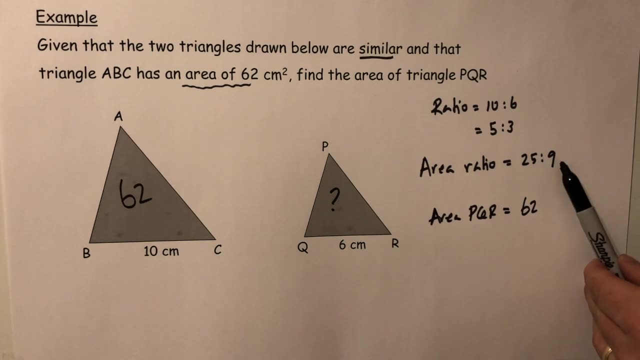 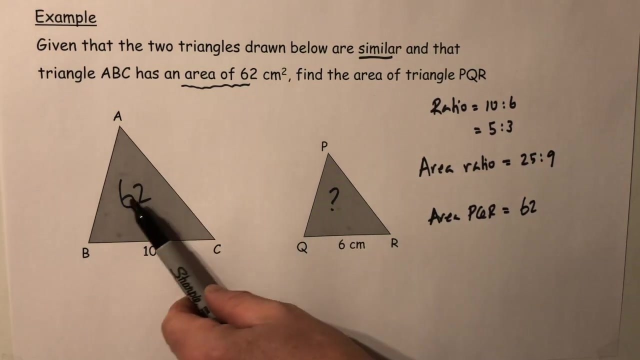 So the area of PQR. it's related to the 62. However, it's either multiplied by 25 over 9, or it's multiplied by 9 over 25.. Now, because this triangle is smaller than this triangle, I need to multiply by 9 over 25.. 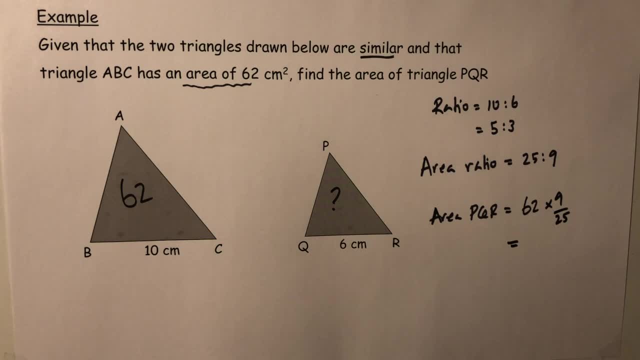 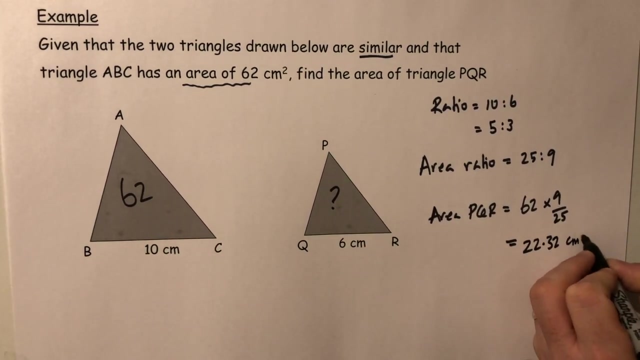 If I was to do it the other way around, I'd end up with a larger area, which is incorrect. So 62. Times 9, divided by 25, comes out as 22.32 units in centimetres. so area centimetre squares.